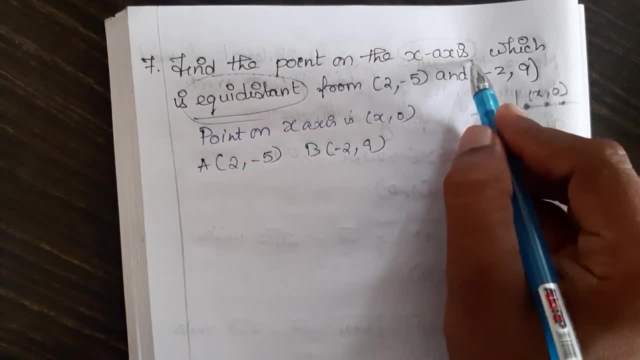 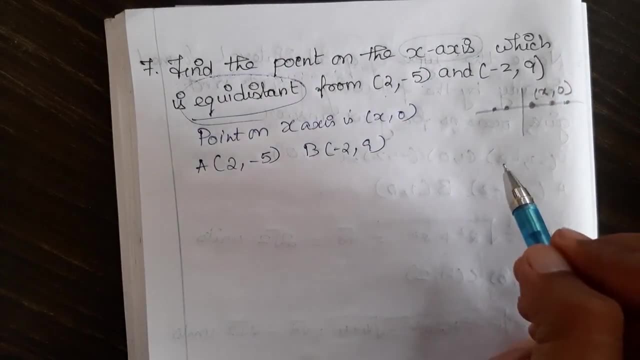 2 comma 9 and given condition it is the equidistance from the x-axis. So from the x-axis 2 comma minus 5, distance will be equal to the distance between the x-axis and the minus 2 comma 5.. That means: 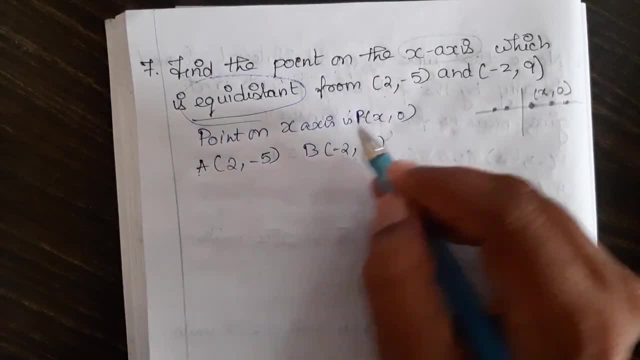 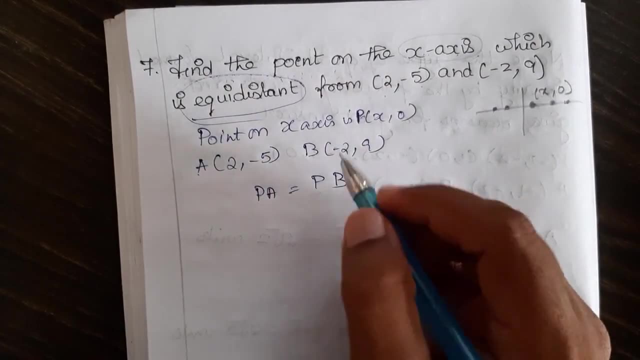 let me call it as a point p. p a will be equal to the p b. So distance of p a will be equal to the p b. That way, that is what they have given: a equidistance. So the p a will be that. so to find the p a, that you consider these two points So 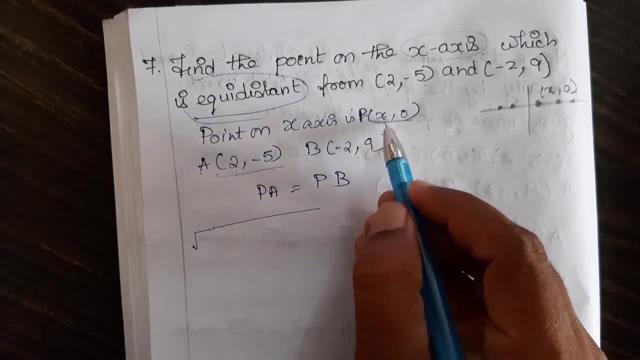 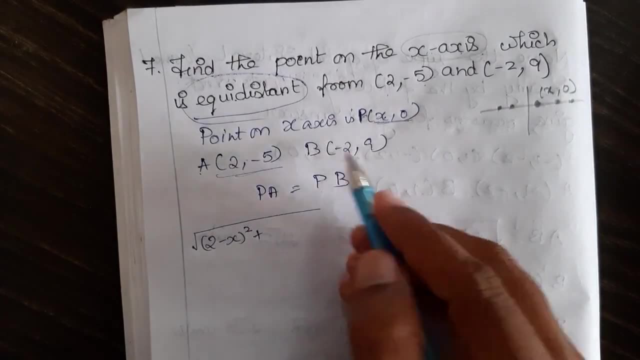 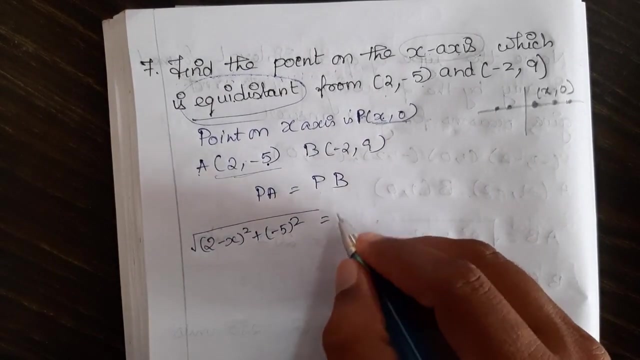 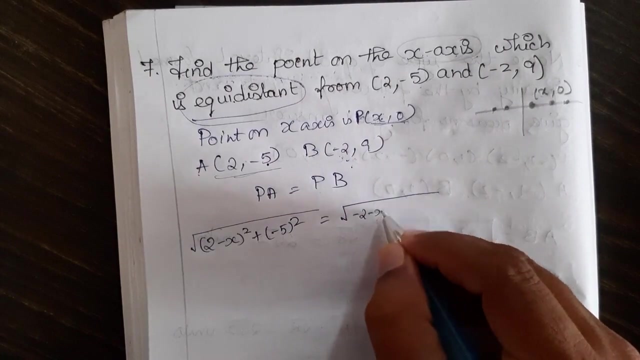 square root of x 2, here is a 2.. 2 minus x, 2 minus x, the whole square plus minus 5 is a 0.. So minus 5, the whole square is equal to 0.. Square root of p: b: Now these two. So here is x: 2 minus 2 minus x, the whole square, plus 9 minus 0. 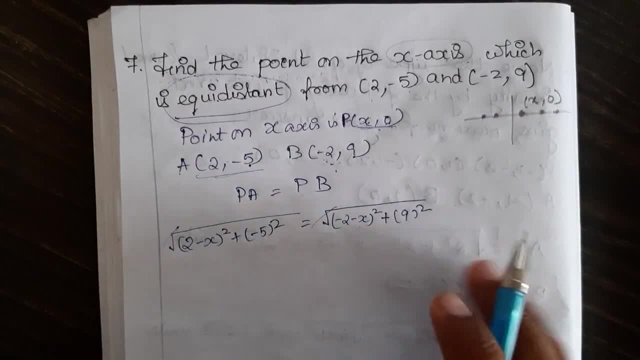 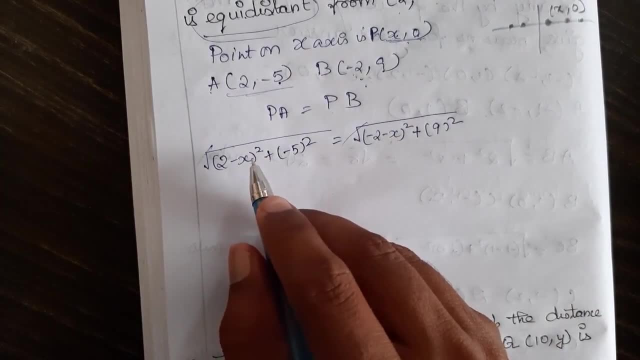 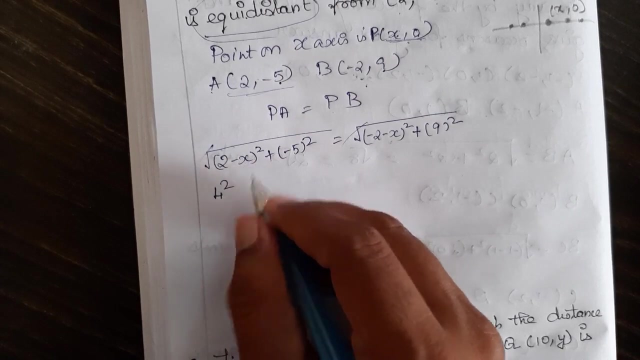 just a 9 square. right So, square root, square root, we can cancel by taking. but since the square, it will become a square and square and square it will be cancelled. right So now this we can expand using the identities. right So 2 square is a 4 square and it will become a plus x square. 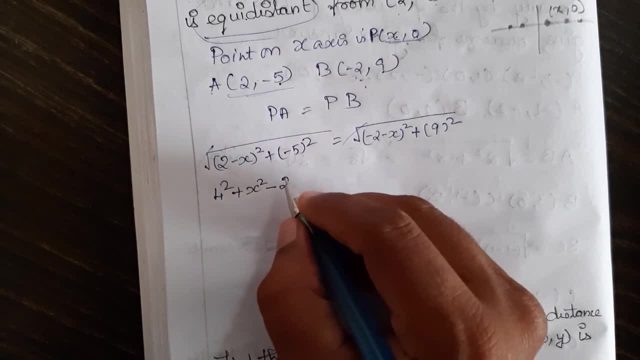 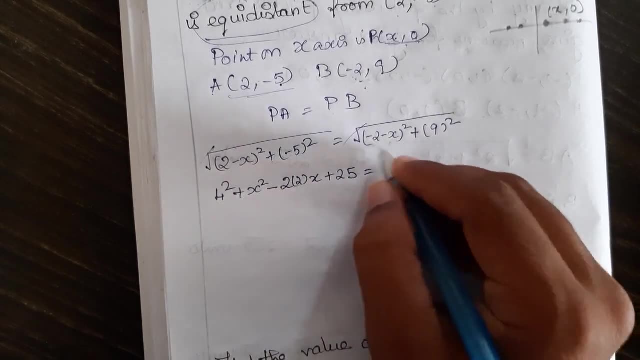 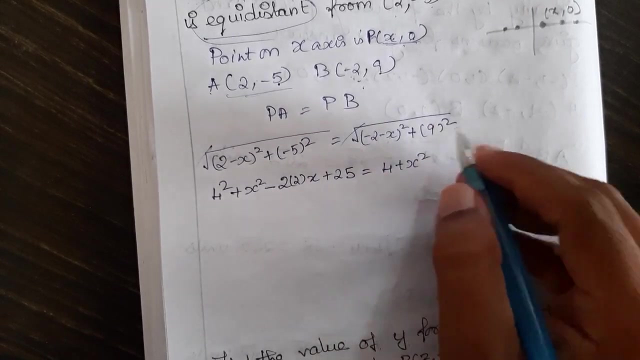 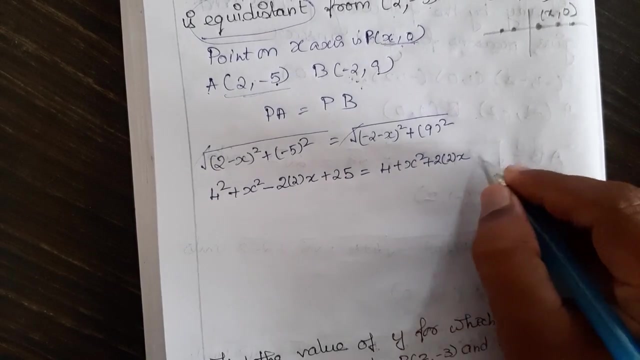 So here minus 2 into 2 into x, 2, a b right plus 5 square is a 25 is equal to. here the minus will be like: a minus 2 square will be the 4 and minus x square will be the x square and plus minus into minus will become 2 right. So 2 into 2 to 2 into x plus 9 is a 81.. 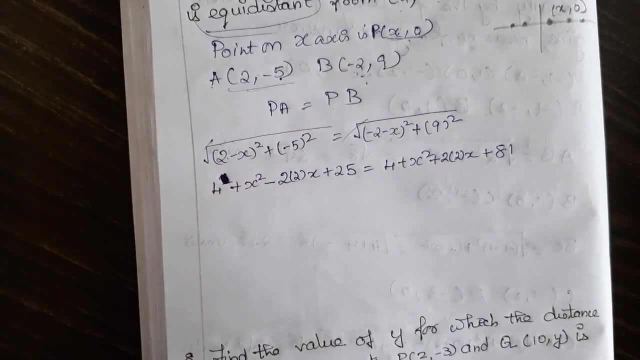 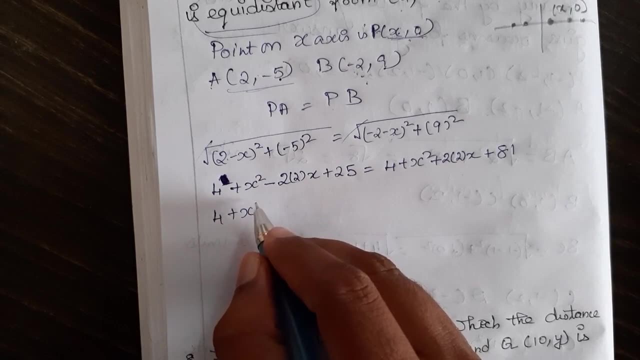 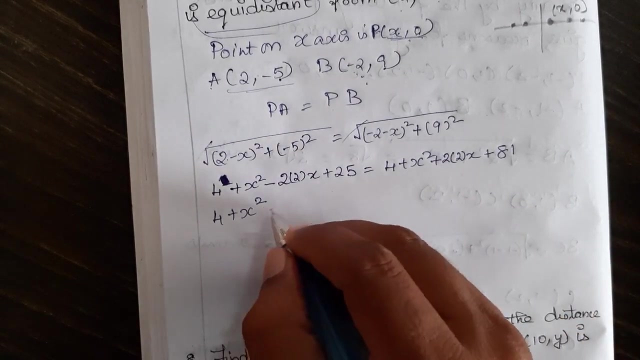 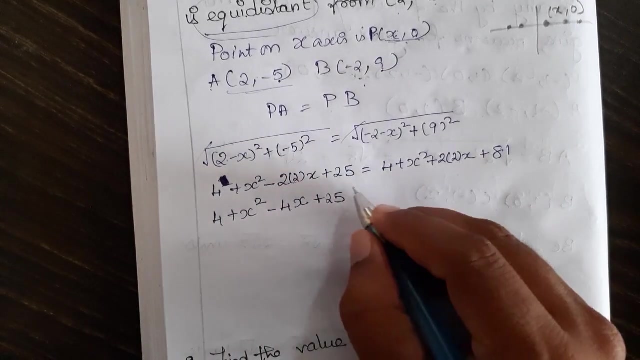 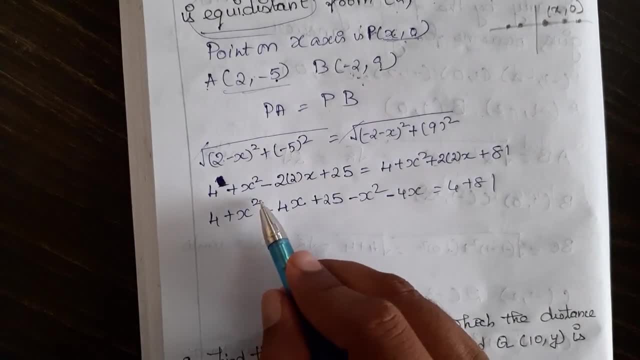 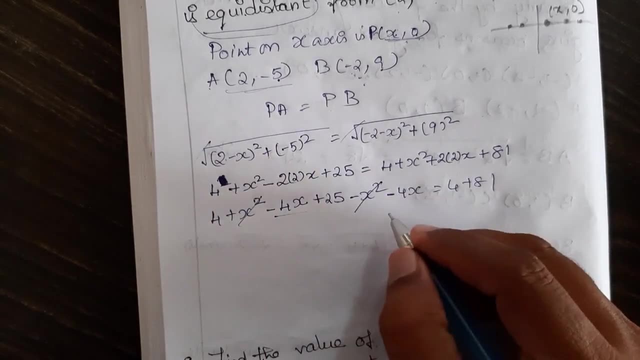 x is equal to 4 plus 81. so plus x square minus x square will be 0, that's 4, and 25 will take this side and minus 4 x, minus 4 x is a minus 8 x. so minus 8 x is equal to 4 plus 81 is a 85 and 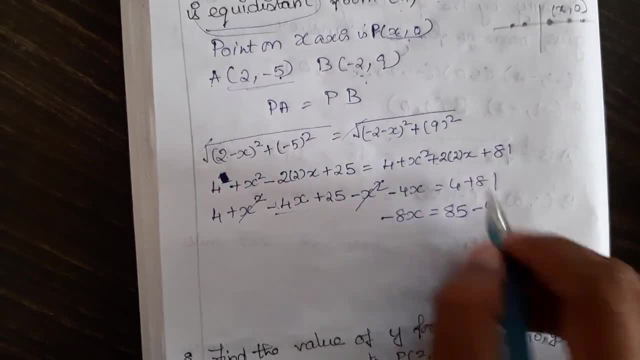 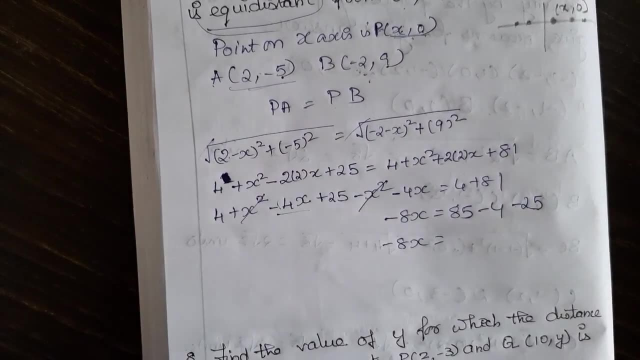 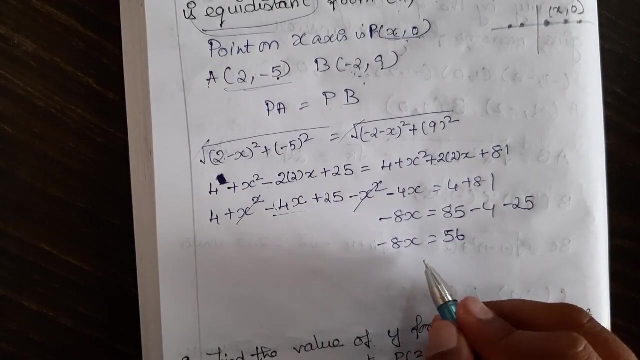 this 4, it will take it will be minus 4 and 25 will be a minus 25. so minus 8, x is equal to 85, minus 4 is 81. 81 minus 25, 56 right and x is equal to 56. divided by minus 8 it will comes for. 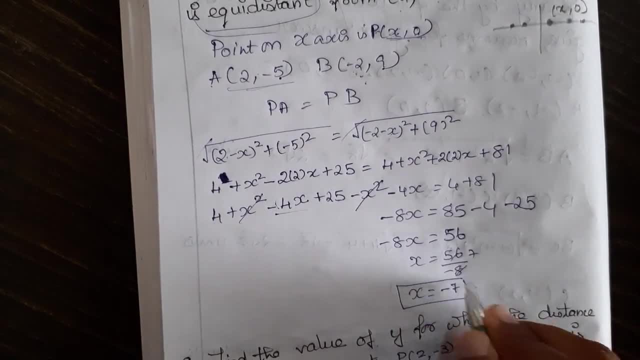 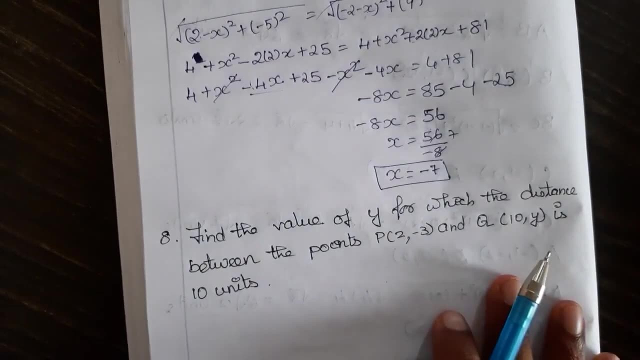 7 times so x is equal to negative 7. so point on the x-axis is that we have found x is a negative 7, so here is equal to minus 7 comma 0, right? so therefore x is equal to minus 7 comma 0, right? so therefore? 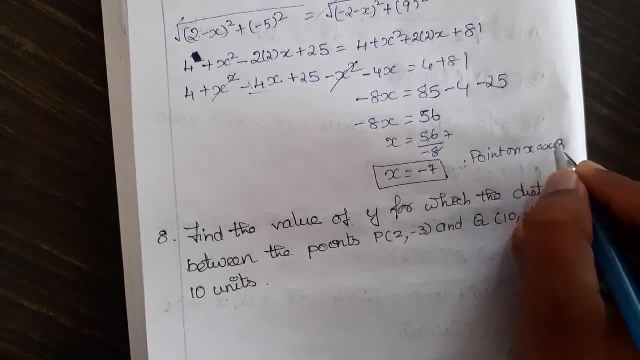 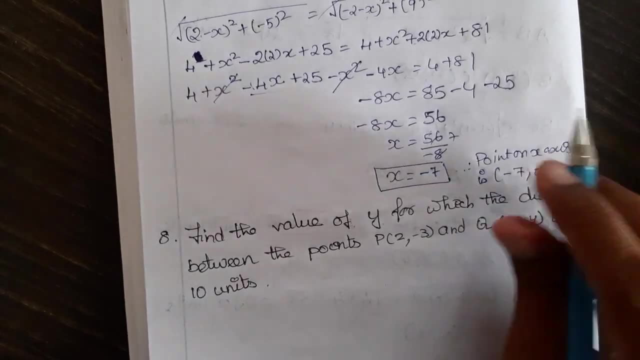 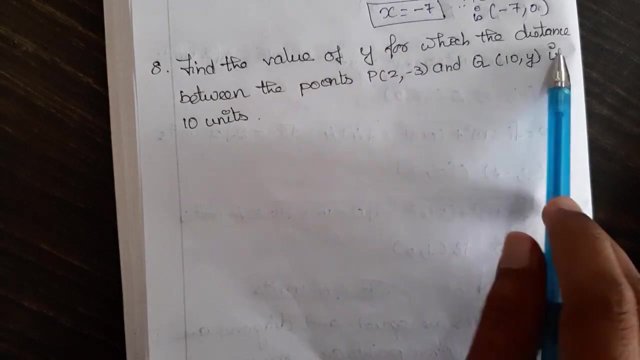 x is equal to minus 7 comma 0, right? so therefore, point on x-axis is minus 7 comma 0. that's why we consider x comma 0 minus 1 comma 0. so here we go for the next problem. find the value of y, for which distance between the point p? 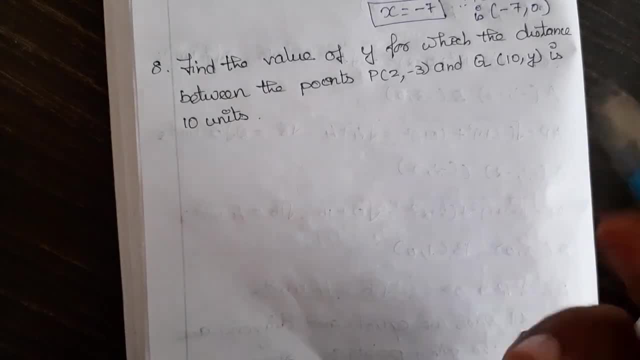 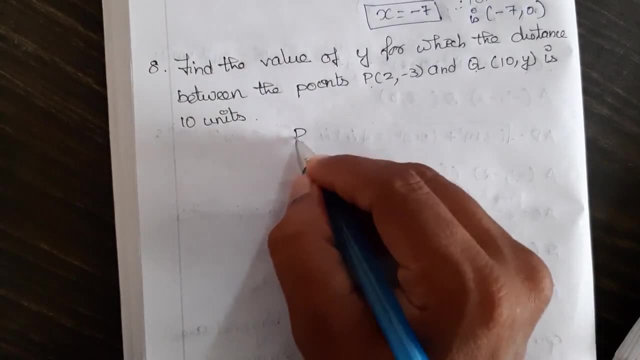 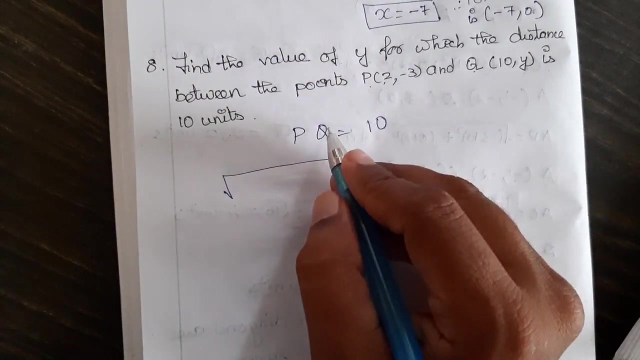 2 comma minus 3 and q 10 comma. y is 10 units. the distance is given. we have to find the value of y, so so distance is nothing. distance between p? q is equal to 10. pq will be written as a square root of x 2 minus x 1. x 2 is a 10 minus 2 is an. 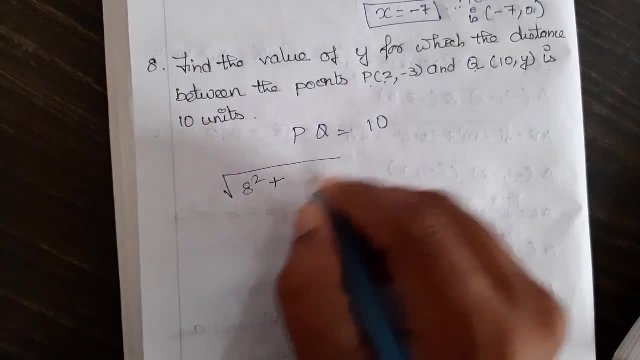 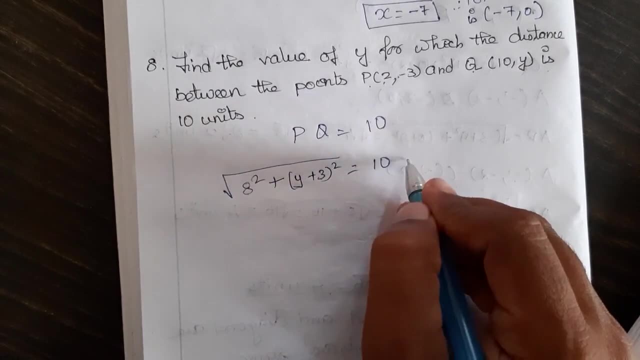 8. so 8 square plus y minus into minus 3 is plus 3. the whole square is equal to 10. if you take square to this it will become a square, and 8 square is a 64. plus this we can use an identities. 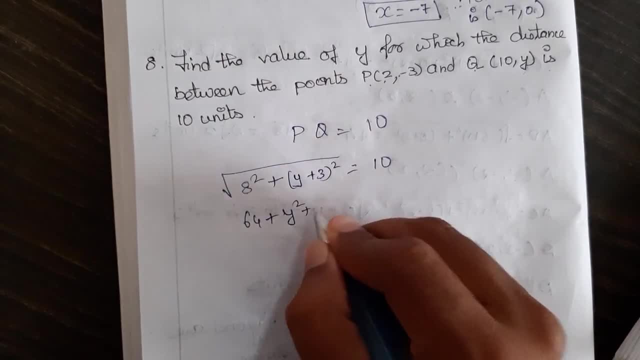 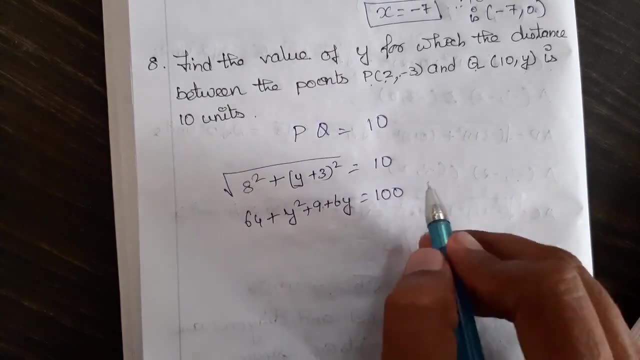 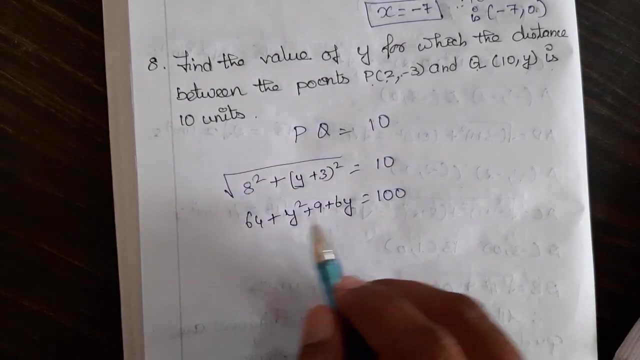 it will become a y square plus 3 square is a 9 plus 3. 2's are 6. 6 y is equal to 100 right. taking square this side, it will become a so square out of this side it will become a square clear. so now we can obtain the 64 and 9. it will be in like in a something. 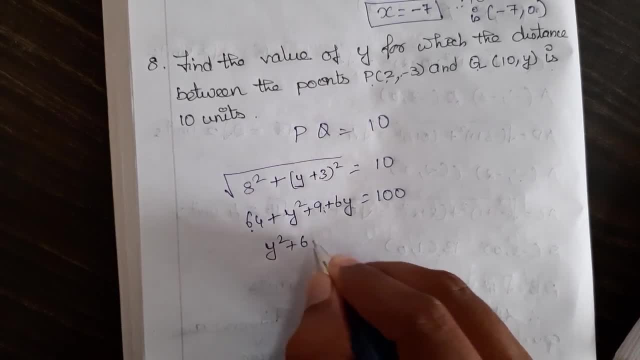 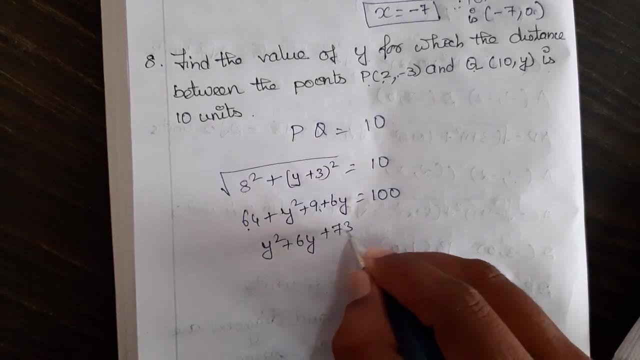 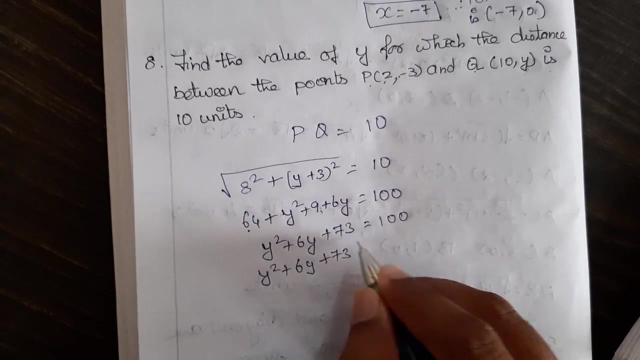 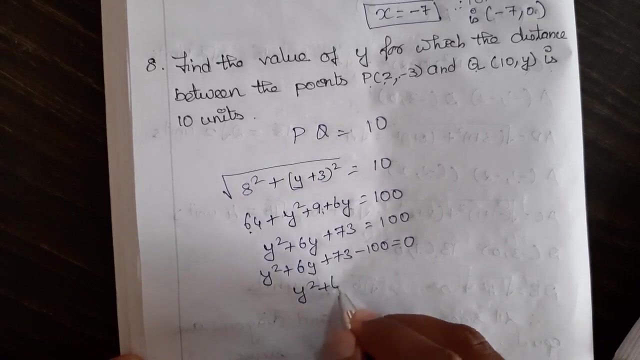 quadratic form right: y square plus 6 y 64 plus 9, 73 is equal to 100. so y square plus 64 plus 73, if you bring under here it is a minus. 100 is equal to 0, and if you subtract we will get a y square plus 6 y 6, 73 minus 100 is a minus. 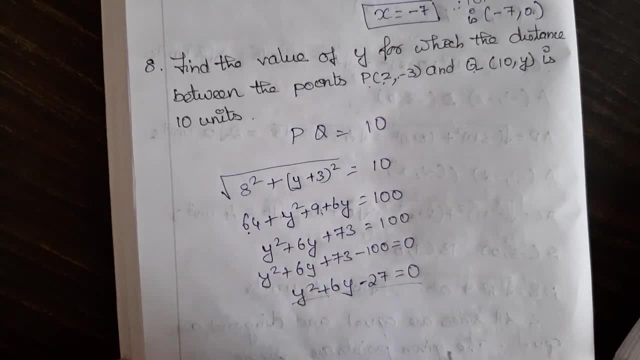 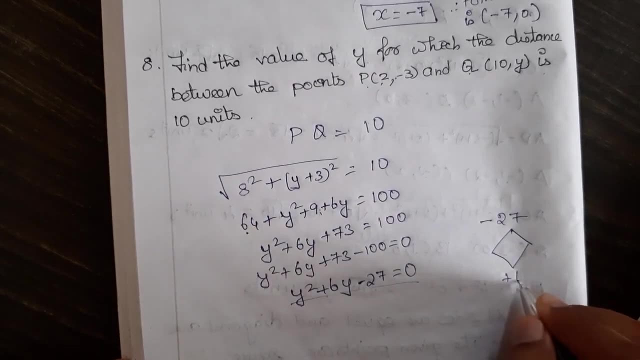 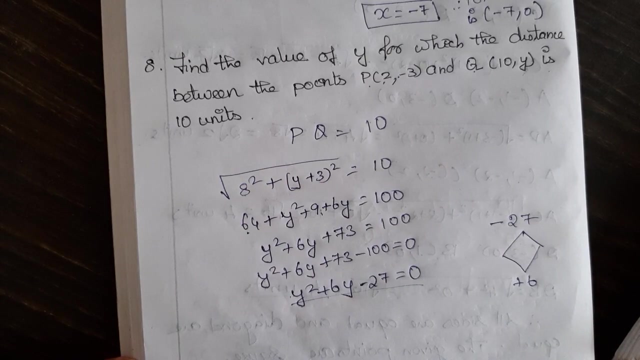 27 equal to 0. now it is a quadratic equation we can solve. so the product is a minus 27 and the sum is a plus 6. so 1 is multiple right. so what we will get, 9, 3 is a 27 and if we subtract 9 and 3 is a 6 right. 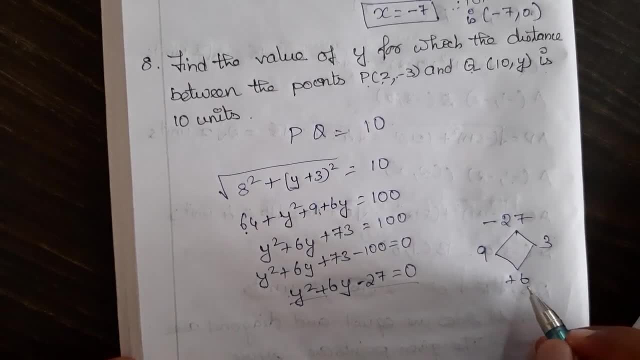 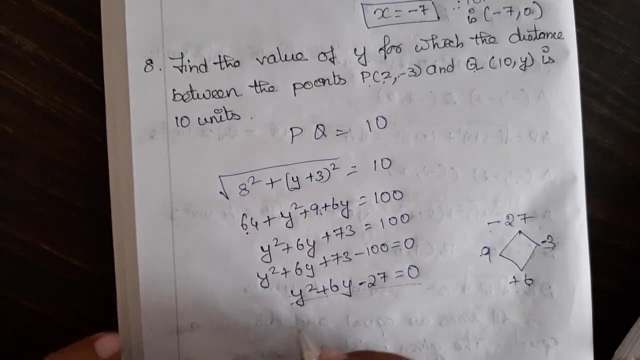 9- 3 is a 27. if you subtract it you have to be a plus 6, so we will make a minus 3 here, right? so 9 into minus 3 is a minus 27. 9 minus 3 is a plus 6. so you divided by the 1 right. 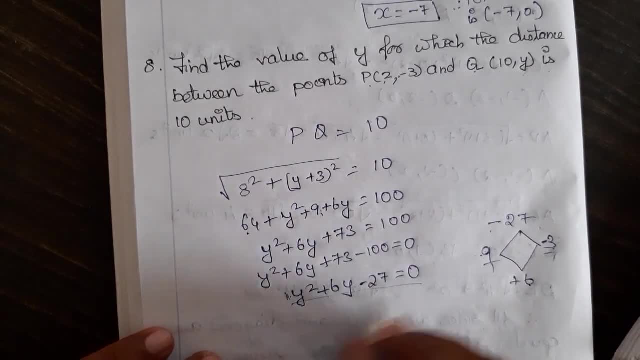 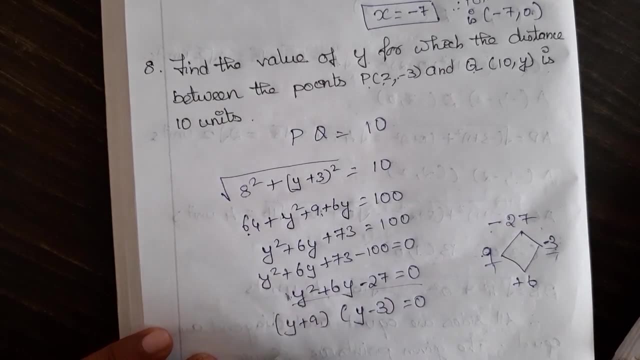 1 only. we have multiplied that. so 1 y, it is a y, right. so y plus 9 into y minus 3 is equal to 0. so y plus 9 is equal means then y is equal to. so consider y plus 9 equal to. 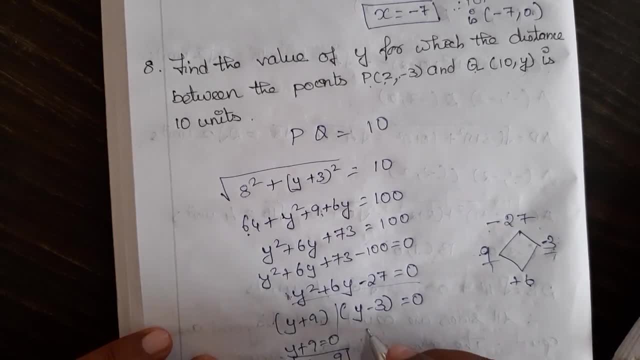 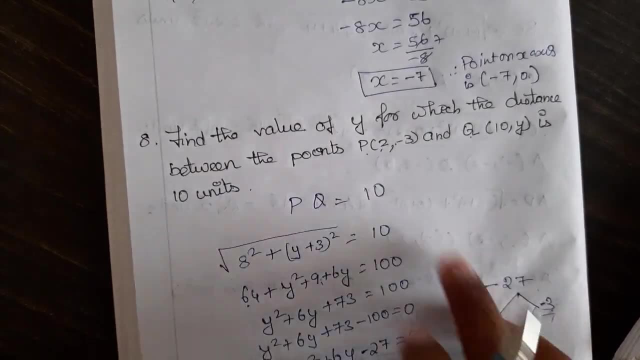 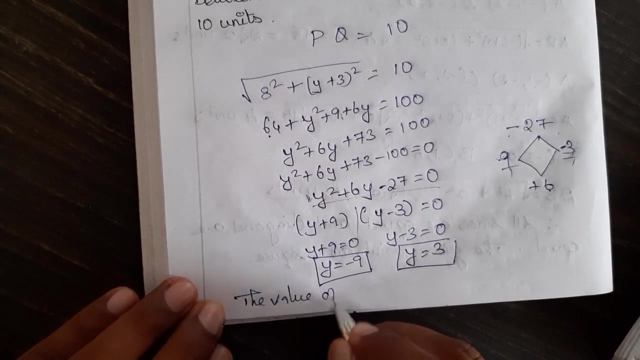 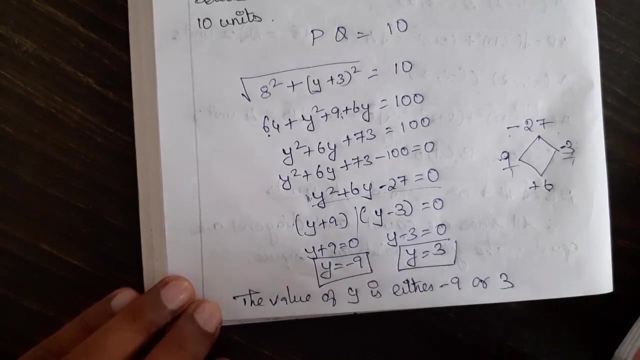 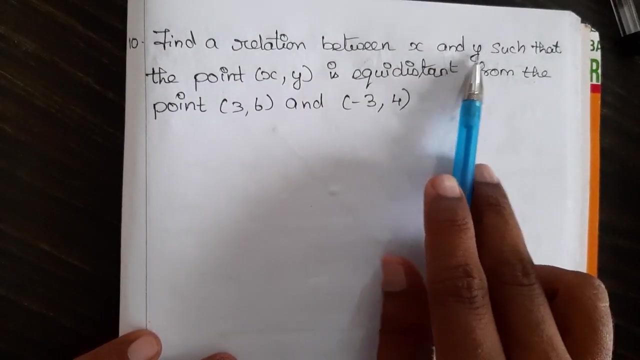 0, then y is equal to minus 9, or y minus 3, equal to 0, then y is equal to 3. so the value of y either minus 9 or plus 3. the value of y is either minus 9 or plus 3. clear, here we go for the next problem. find relationships between x and y such 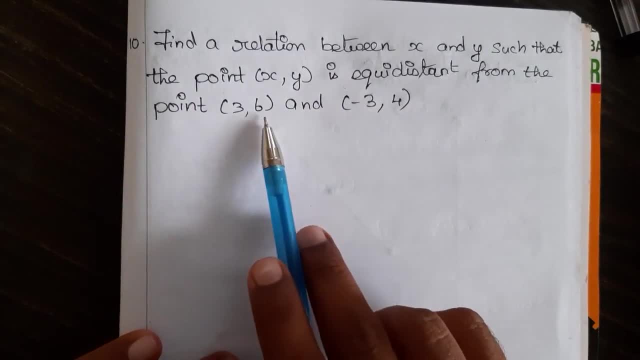 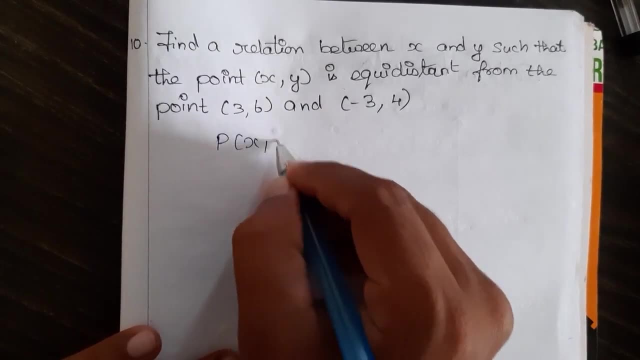 that the point x comma y is equidistant from the point 3 comma 6 and minus 3 comma 4. so it is, let me consider this point as p, p, x is a x comma y and the equidistant point is a 3 comma 6 and b. 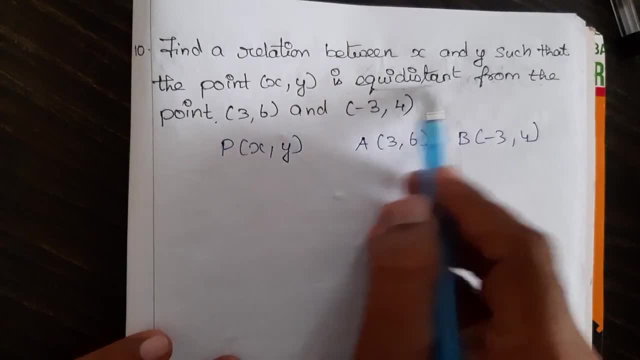 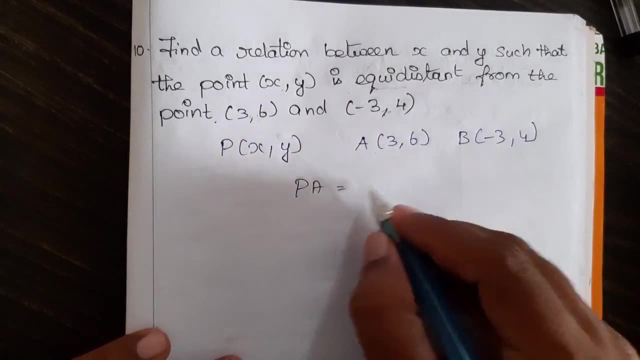 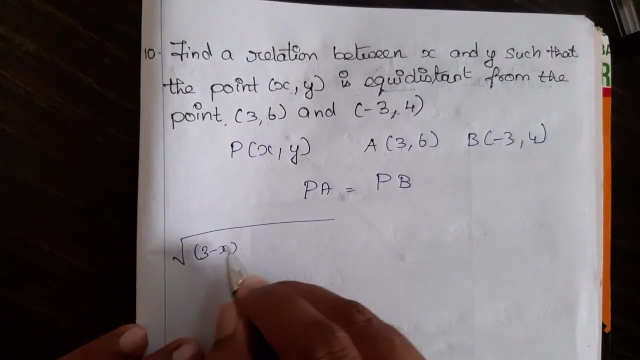 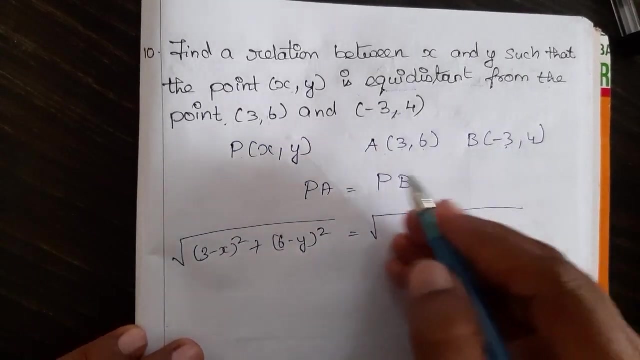 minus 3 comma 4. so it is given a equidistant distance from this. distance between these two points will be equal to distance between these two points. that is nothing. but PA is equal to PB. So PA is a square root of 3 minus x square plus 6 minus y square is equal to. PB is equal to minus 3 minus x square. 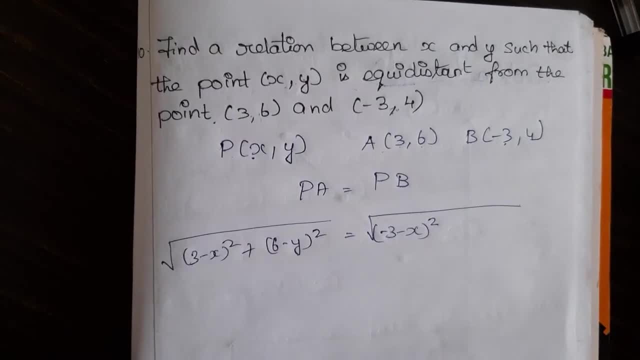 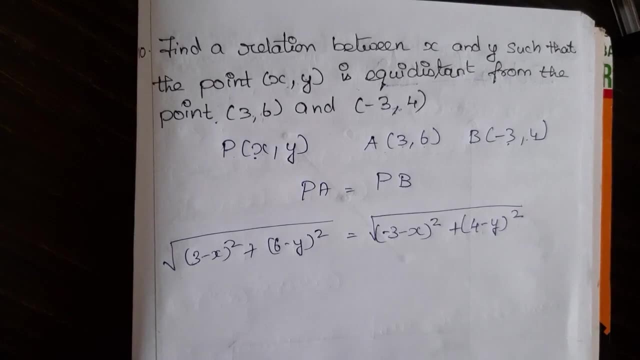 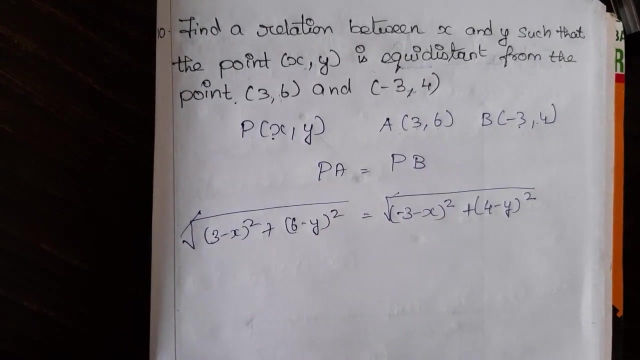 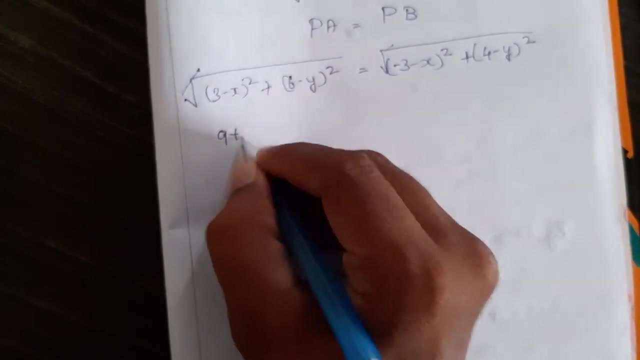 So plus 4 minus y the whole square And square and square root will be cancelling. So 3 minus y the whole square. we are using an identities. So 3 minus x the whole square is a 9.. 3 square is 9 plus x square is x square minus 3 to the 6.. 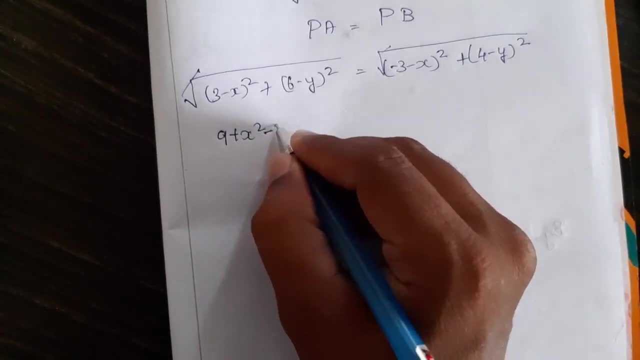 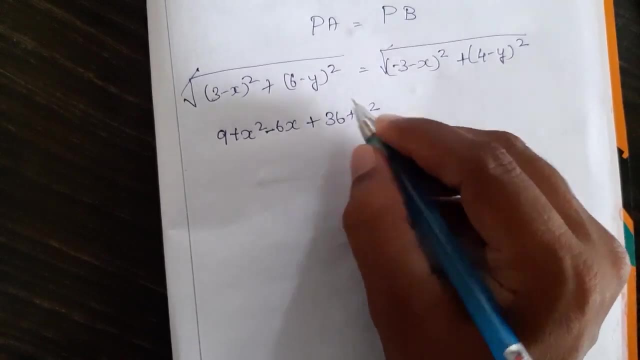 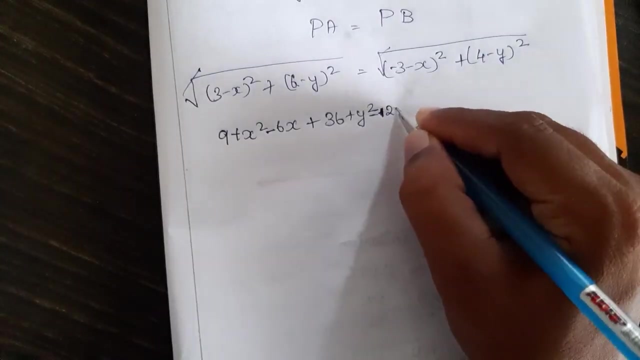 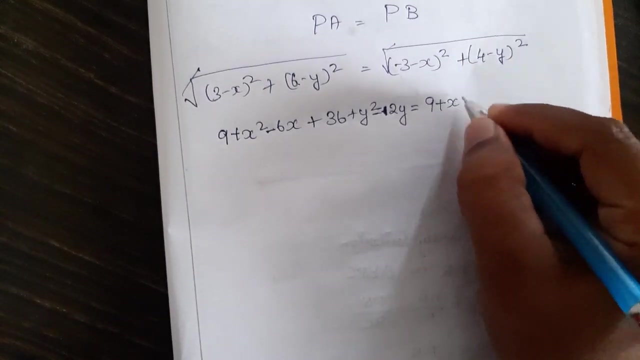 6 and x is a 6.. Minus 6x plus, here the 6 square is 36 plus y square and 2: 6 are 12. it's a minus minus 12. y is equal to the same. here minus 3 minus x square will become 3. square is a 9 plus x square plus 6x. 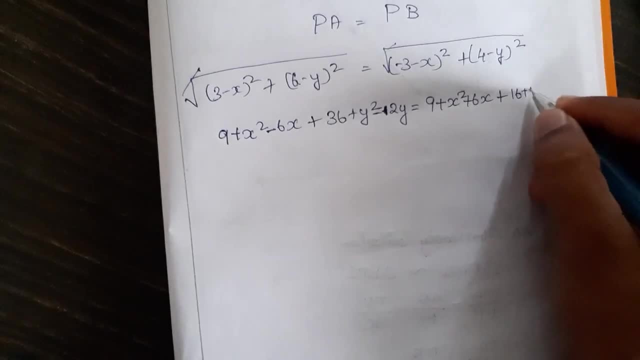 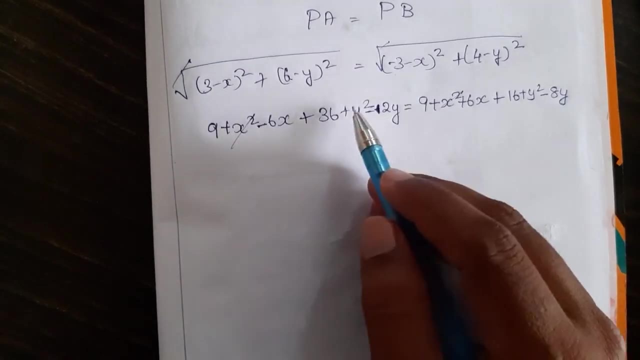 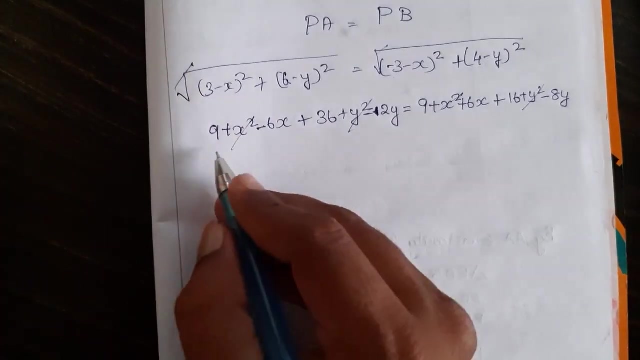 plus here, 4 square is 16 plus y square minus 8 y right. so x square and x square will be cancelled, while bring this, it will be subtraction and y square and y square also will be a 0. so let x and y term be here. let me bring everything here. we need only relationship, right? 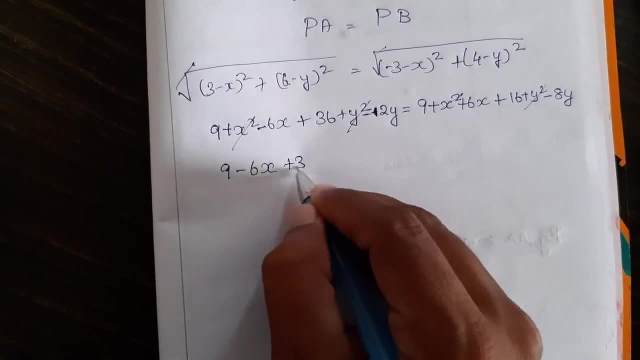 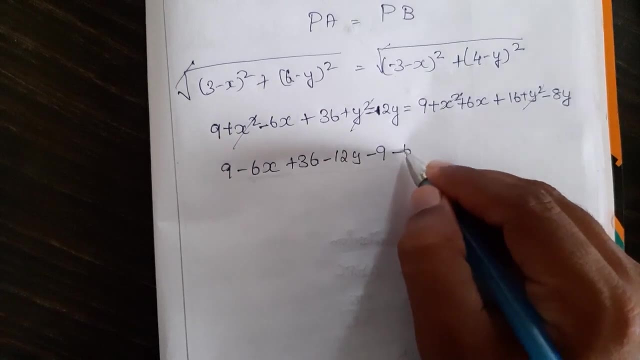 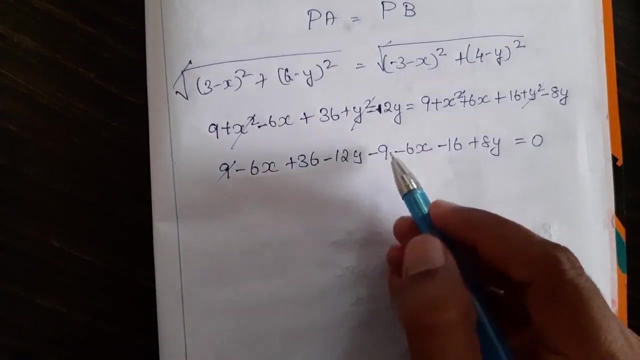 so 9 minus 6x plus 36 minus 12 y, if you bring here it is a minus 9 and minus 6x minus 16 plus 8y is equal to 0. again, the plus 9 and minus 9 is 0 minus 6 and minus 6 is a minus. 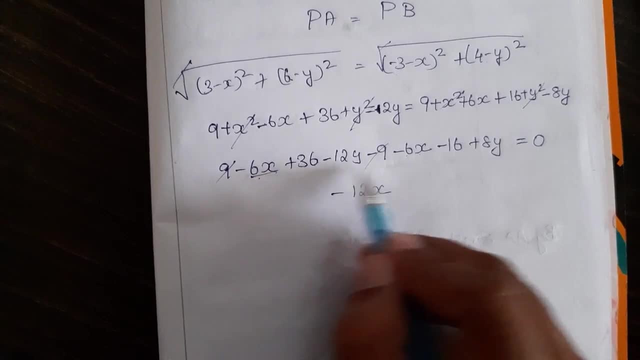 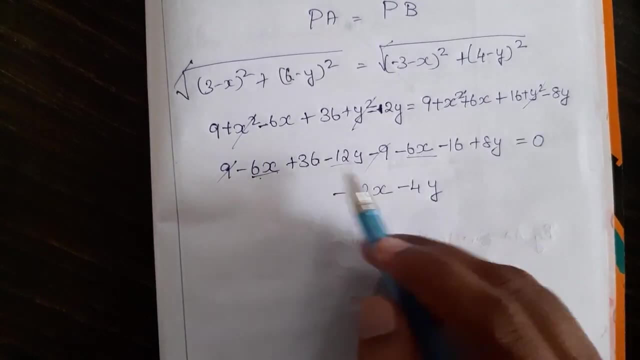 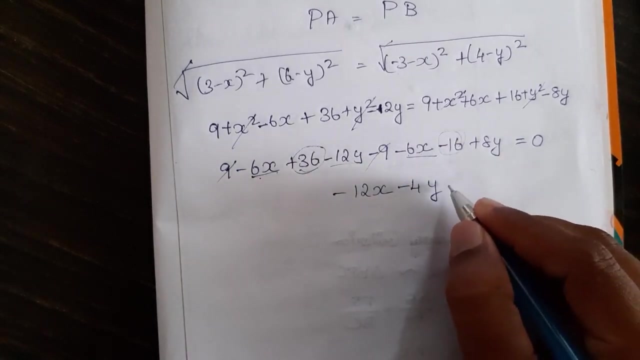 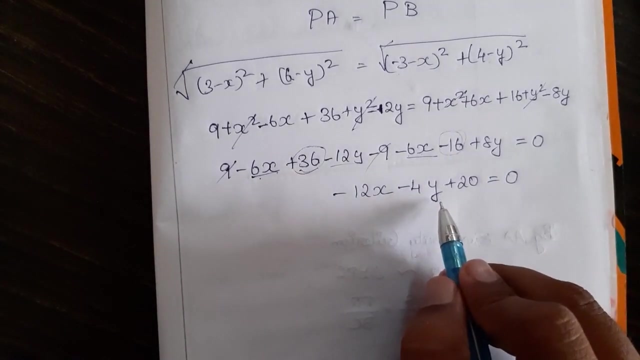 12x. what about the y? so x? 6? u term written: minus 12 plus 8 is a 4 and minus 4 right minus 4y. and at 36 plus 36 minus 16 is a plus 20 plus 20 is equal to 0. okay, i think we can divide the everything with the. 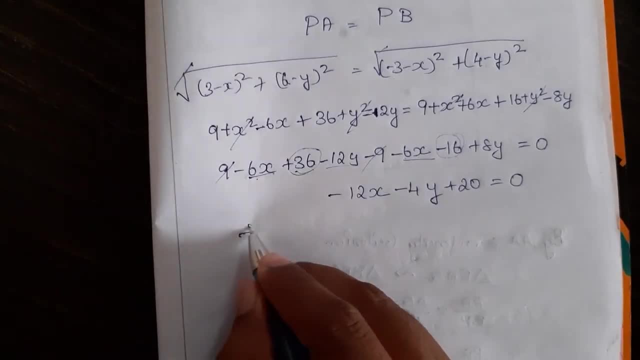 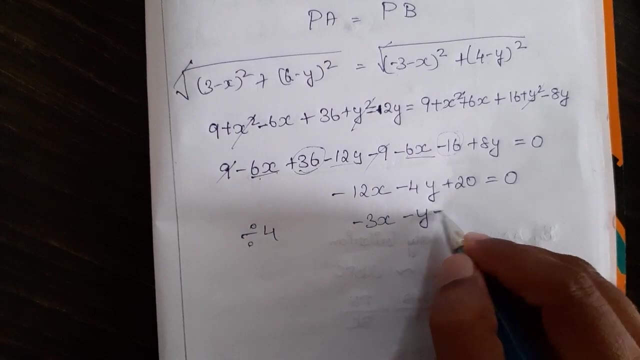 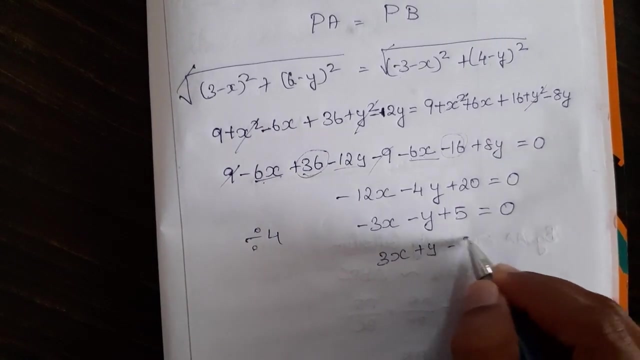 4 table right. divided by the 4 we will get a minus 3x minus 1y plus 5 is equal to 0, or else in the minus also we can change that there's a 3x plus y minus 5 is equal to 0.